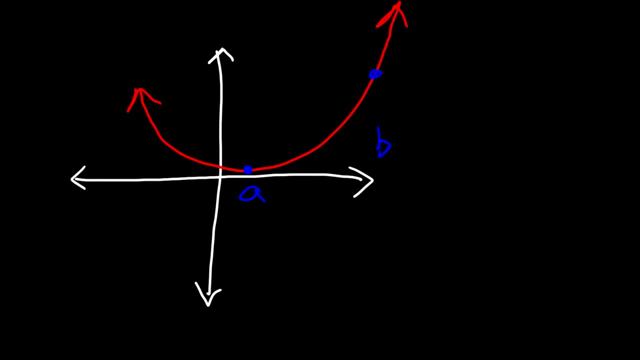 between points A and B, So that's on the interval A comma B, The average rate of change. it gives us the slope of the secant line, And a secant line touches two points on a graph. A tangent line only touches one point on a graph, So that would be a tangent line. 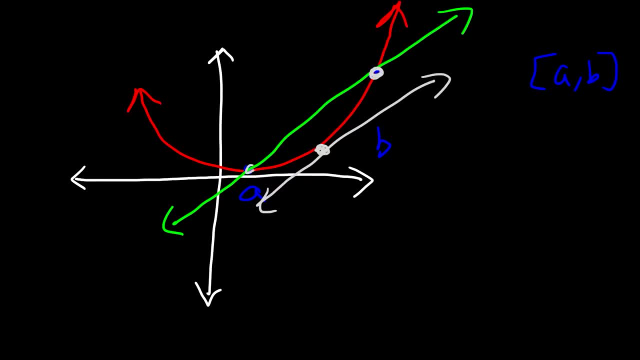 So keep that in mind. The average rate of change represents the slope of the secant line. Number two: calculate the average rate of change of f of x equals x cubed minus 4, from x equals 2 to x equals 5.. So it's going to be f of B. Well, first we need to know what A and B. 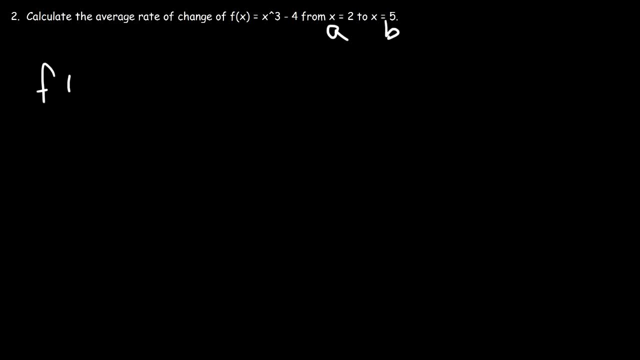 are: A is 2.. B is 5.. So it's f of B minus f of A over B minus A. That's the average rate of change. So this is going to be f of 5 minus f of 2, divided by 5 minus 2.. 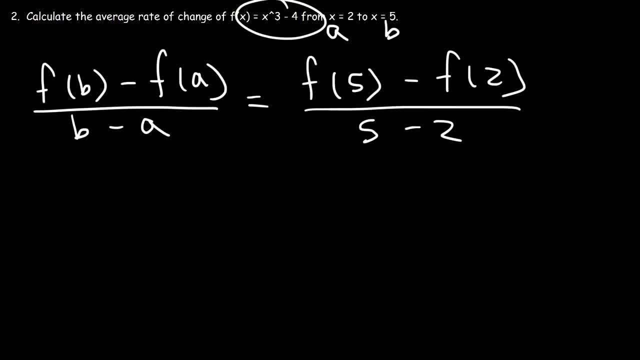 So to calculate f of 5, we just got to plug it in to that formula, So that's going to be 5 to the third minus 4.. And to calculate f of 2, it's going to be 2 to the third minus 4.. And 5 minus 2 is 3.. 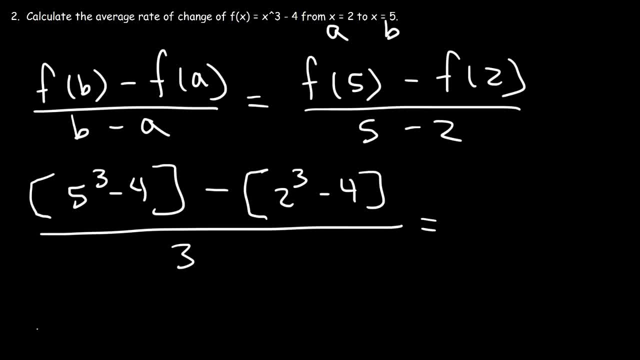 Now, what is 5 to the third power? 5 to the third power, that's 5 times 5 times 5.. 5 times 5 is 25.. And 25 times 5 is 125.. Now 2 to the third, that's 2 times 2 times 2, which is 8.. 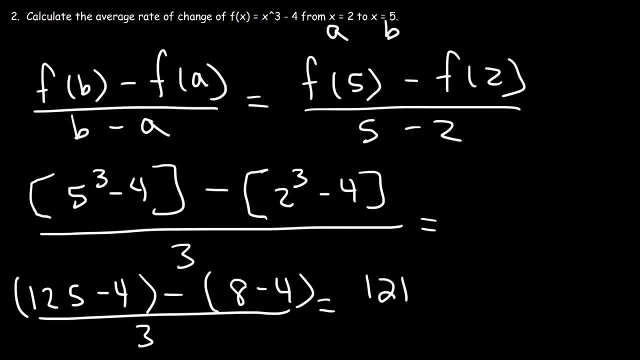 125 minus 4 is 121.. 8 minus 4 is 4. And 121 minus 4 is 117.. So it's 117 divided by 3.. And 117 divided by 3 is 39.. So 39 is the average rate of change. 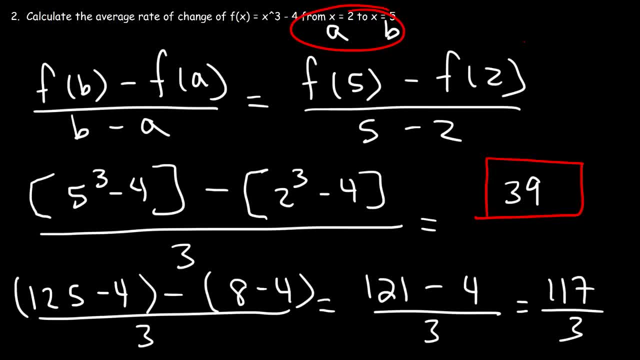 from 2 to 5, or in the interval 2 comma 5.. So now you know how to calculate the average rate of change of a function. So if you want to find more videos on pre-calculus, algebra or even calculus, check out my channel. You can find a lot of other videos that.